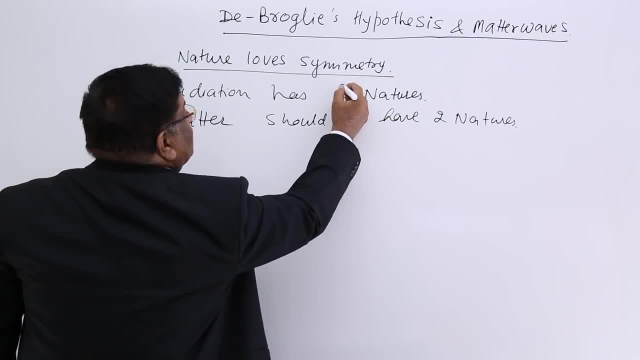 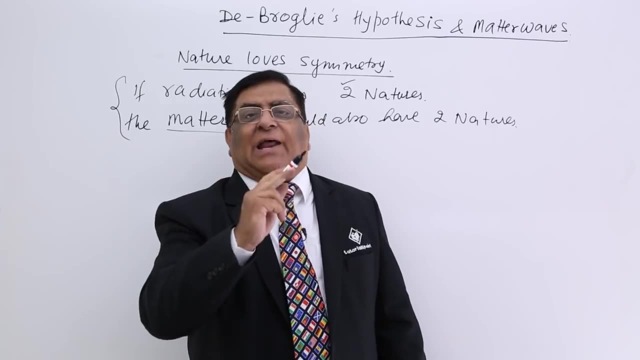 He said: no, The matter also has wavelength, and we don't know about it. symmetrical, the radiation has two natures, then why matter should not have two natures? It should go straight as well as it should go in waves. 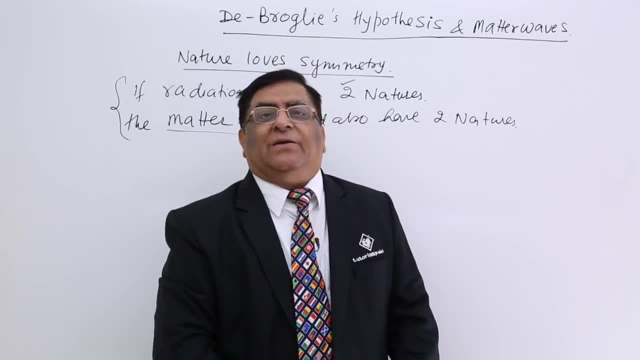 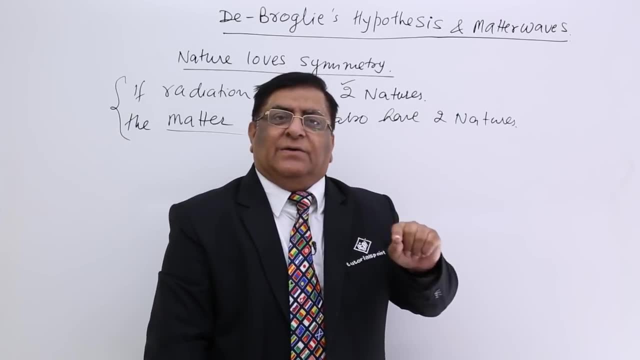 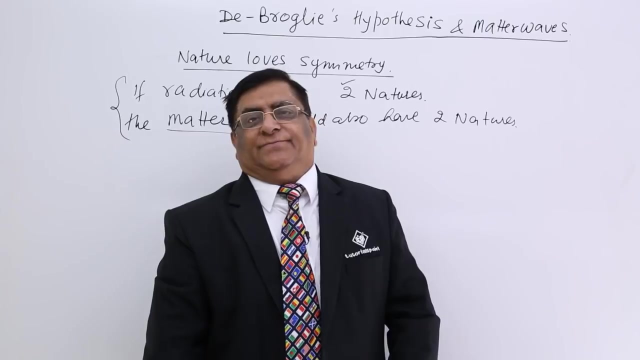 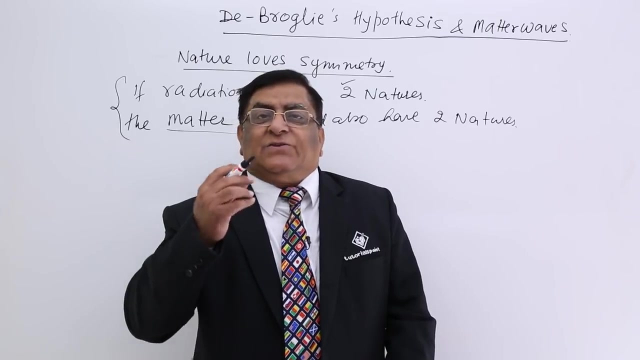 So, on the basis of this thought, de Broglie made an hypothesis, and that hypothesis is that a material, when it is moving, sometimes it acts like a matter and sometimes it acts like a wave. In other words, when a matter moves, then it is always surrounded by, it is guided by, 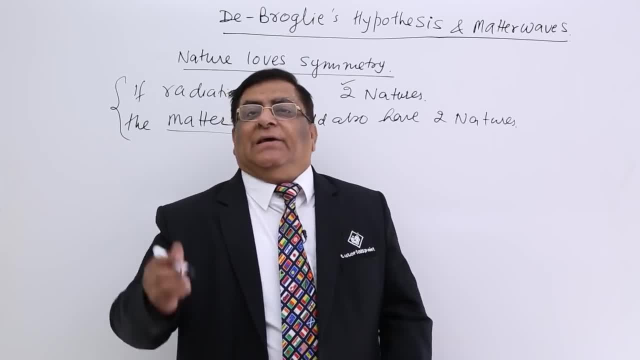 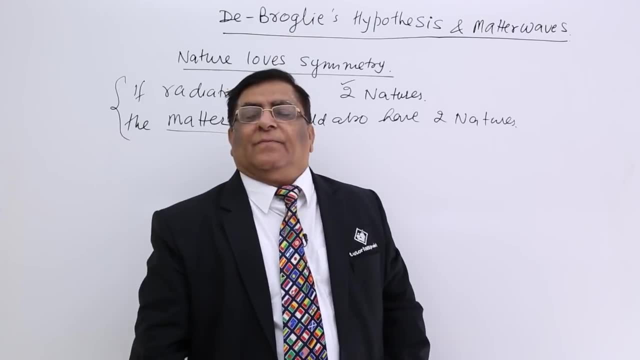 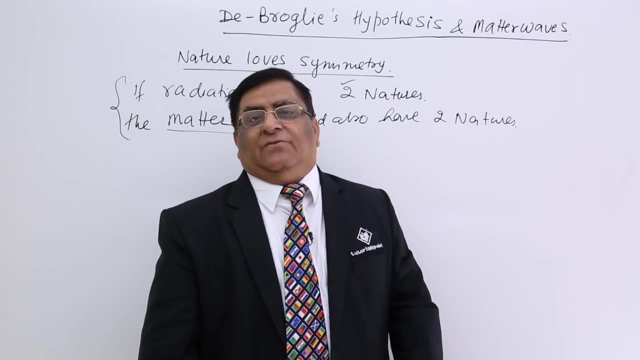 a wave, Again a matter. when it moves, it is guided by a wave which is surrounding it, and that wave is a wave which we have not heard so far, Which we have not learnt so far, and the name of that wave was given as matter: wave. 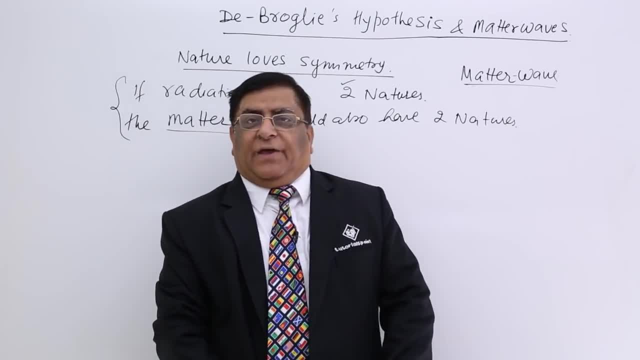 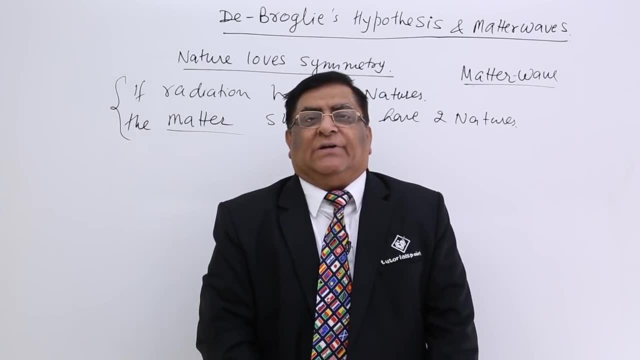 What is a matter wave? Matter wave is a wave which accompanies a moving matter. Is it a material wave? We have learnt that sound is a material wave and there are two type of material waves: longitudinal as well as transversal. He said no. 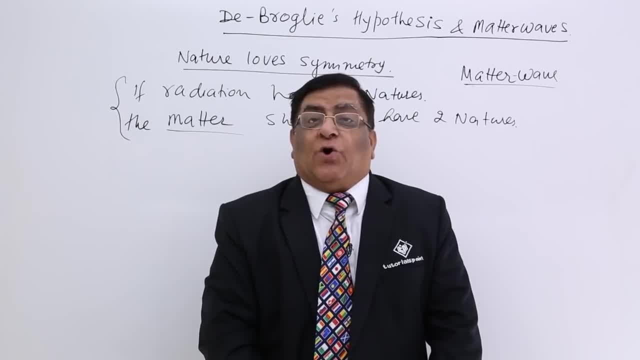 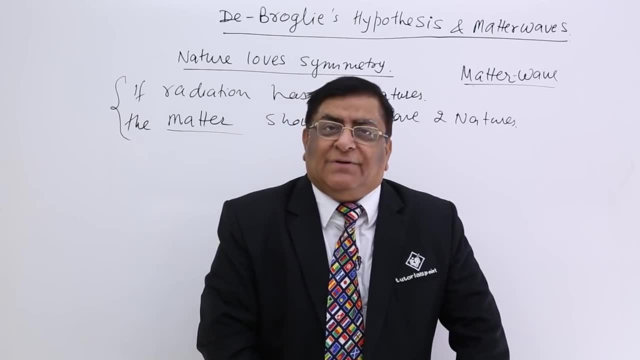 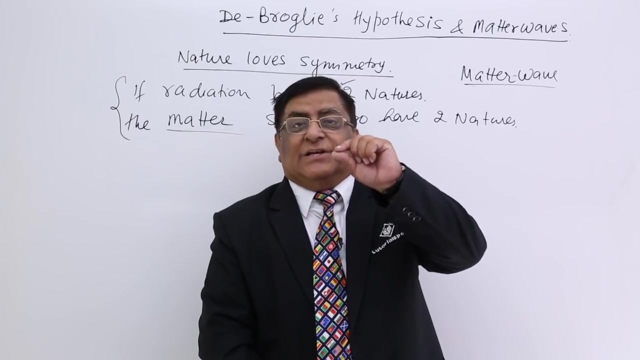 It is not that made by the vibrations of matter. It is not made by the vibrations of matter. Then is it an electromagnetic wave Made by electric fields and magnetic fields, which is created by acceleration or oscillation of electrical charge? He says no. 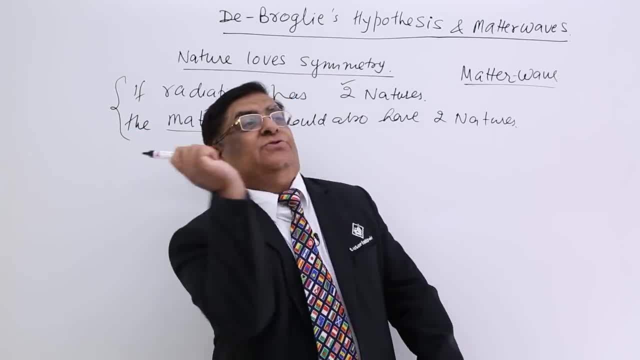 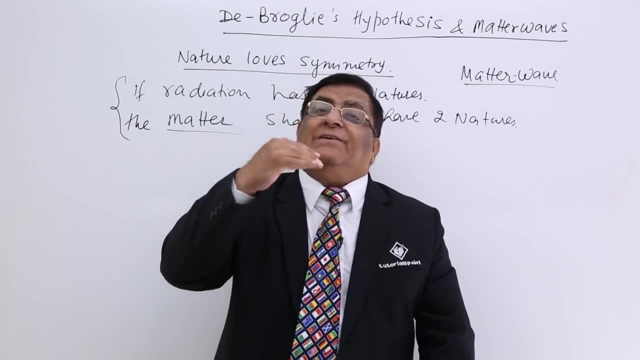 Even if a neutral material moves, even if I throw it, and it moves, a wave guides it. There is a wave that is moving. There is a wave that is moving. There is a wave that is moving. It is connected on it and it is a different type of wave. 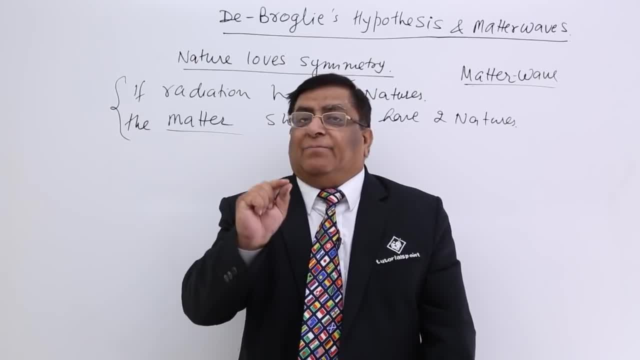 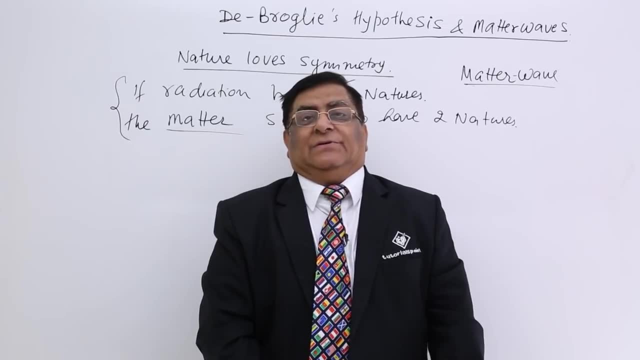 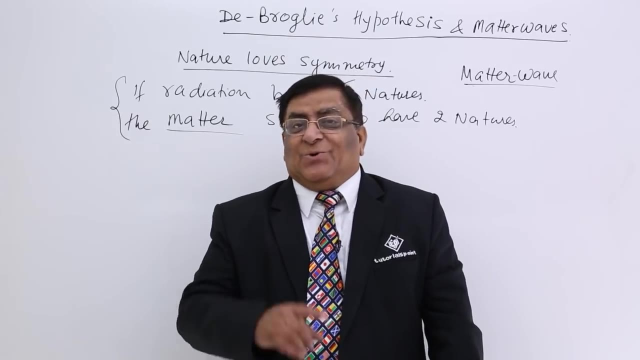 Neither the wave made by the particles nor it is an electromagnetic wave. It is a third type of wave, That is, material wave. So that was a third type of wave And now, a days, you have seen the news about fourth type of wave. 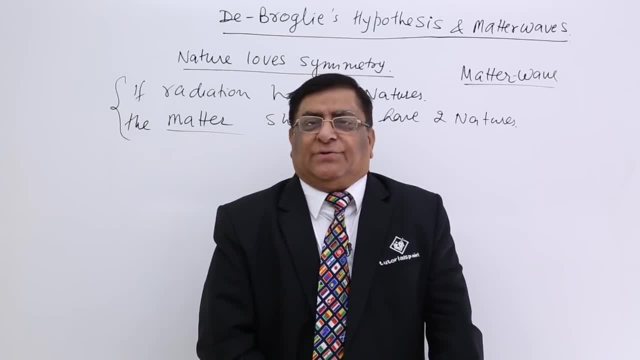 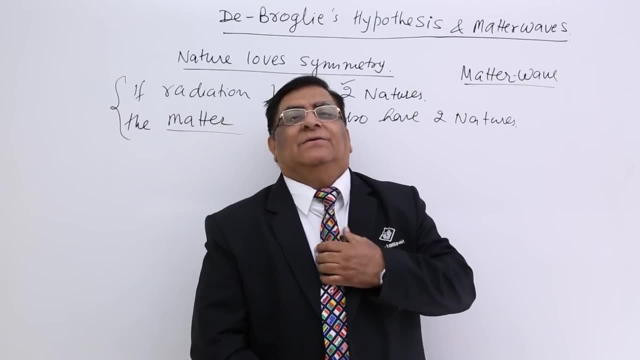 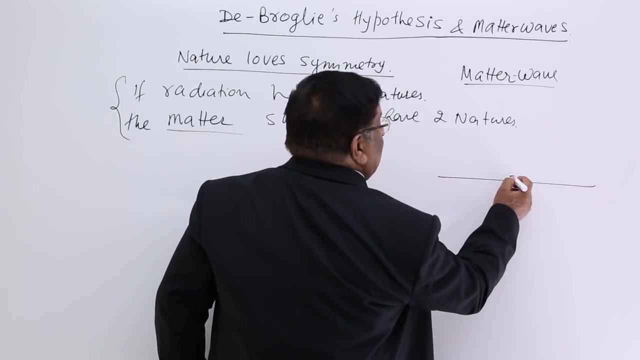 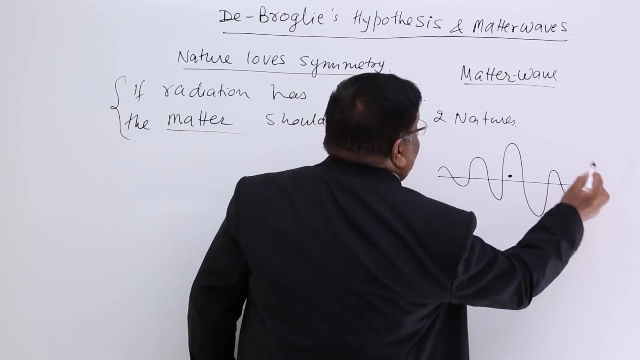 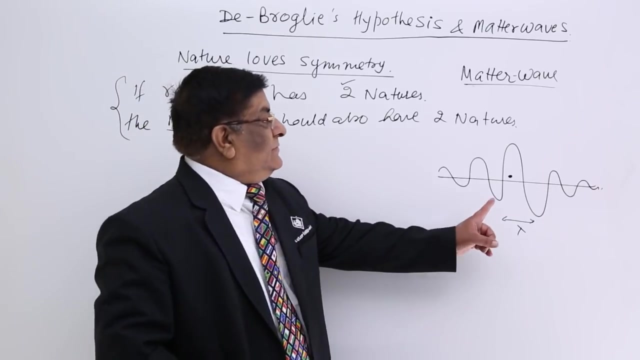 That is gravitational wave. Okay, We are not going to that. Okay, So what de Broglie said is a material wave that guides the motion of a matter, and he says that every moving particle is surrounded by a wave. This wave has got a particular wavelength. 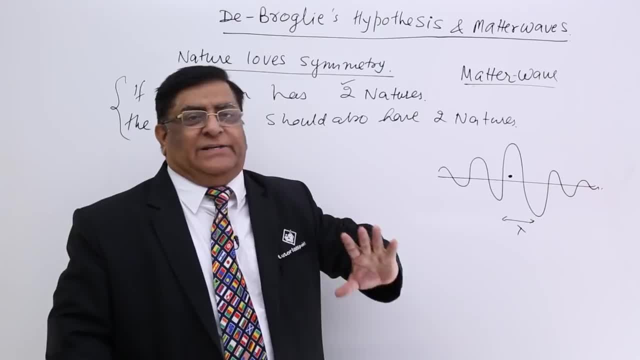 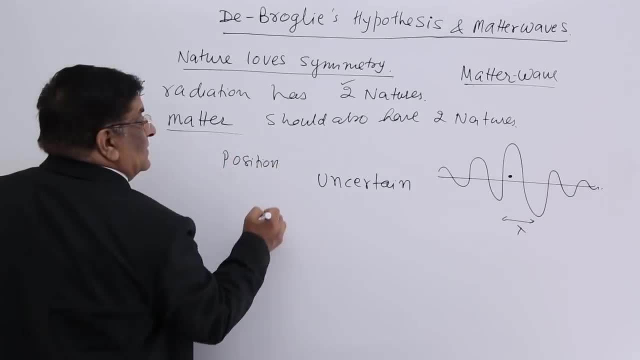 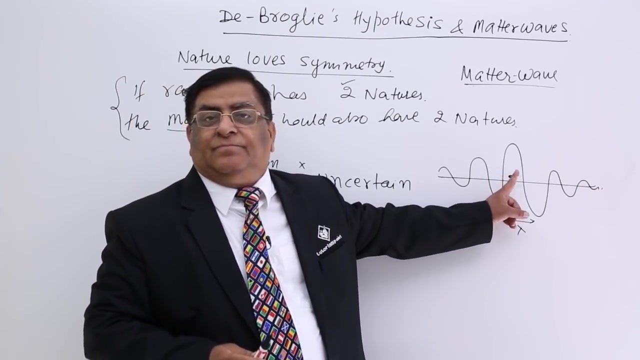 Where is this matter in this wave? It is not decided, It is uncertain. This material has got two things: One is position and other it has momentum: p, position x. So the position and momentum is uncertain. Both the things are uncertain. 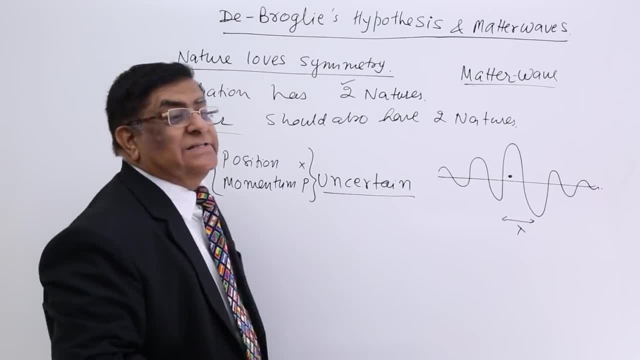 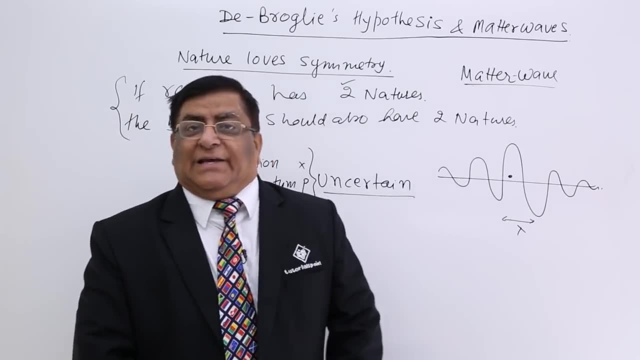 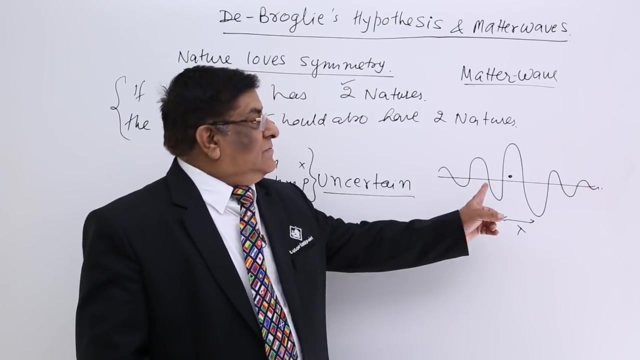 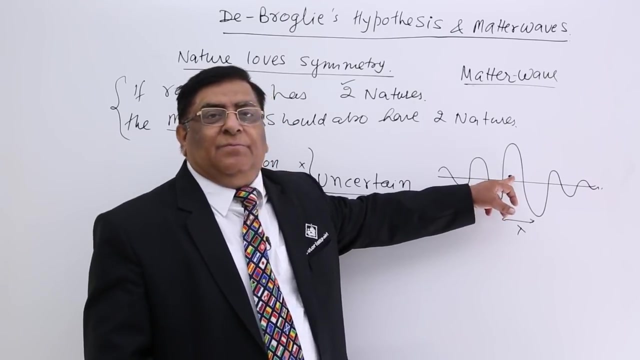 And this is given by the uncertainty principle. These are guided by the uncertainty principle which says, at any time, these two will remain uncertain. The matter wave is a new concept for us, and it says the behavior of this particle will be in the form of waves. 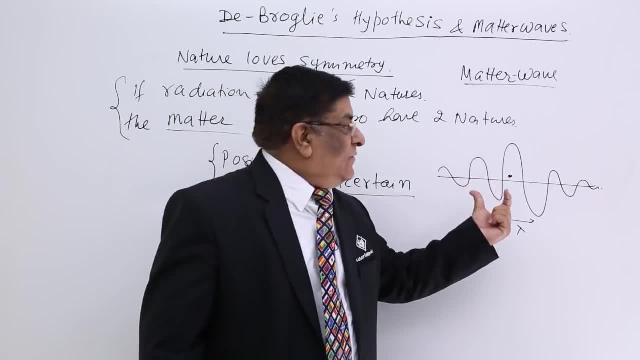 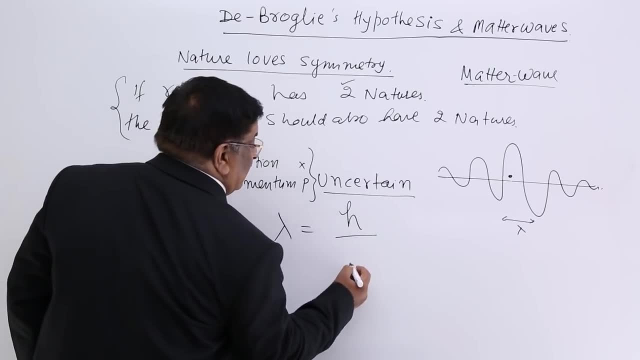 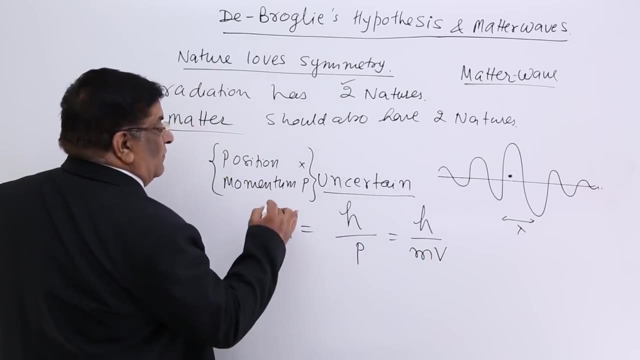 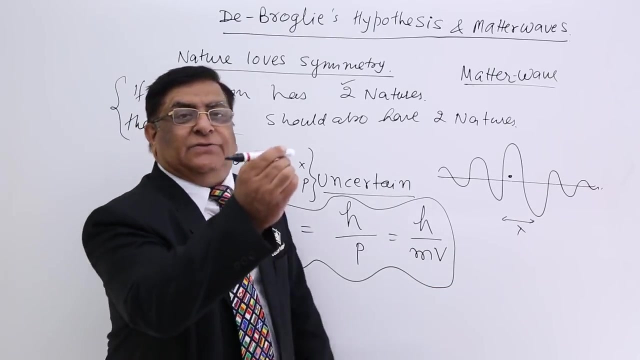 Okay, So this is a wave and that wave will have a particular wavelength, and that wavelength will be given by Planck's constant divided by momentum, Planck's constant divided by mass into velocity. This is what de Broglie says: that if I throw this pen with certain velocity it has a mass. 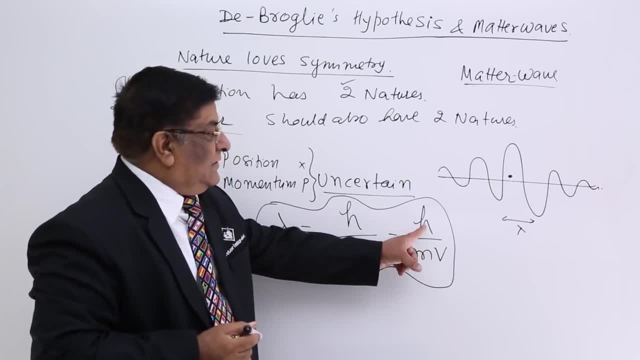 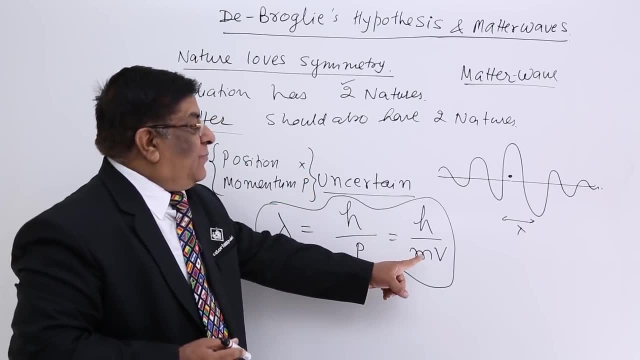 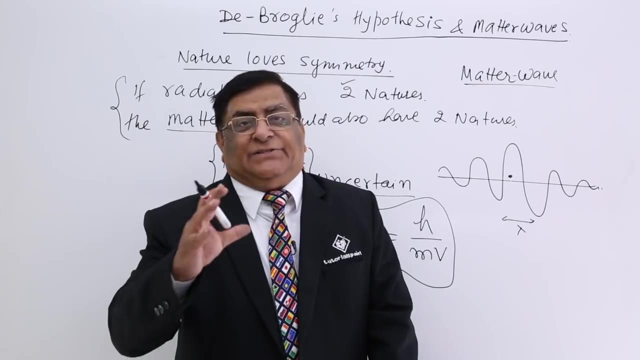 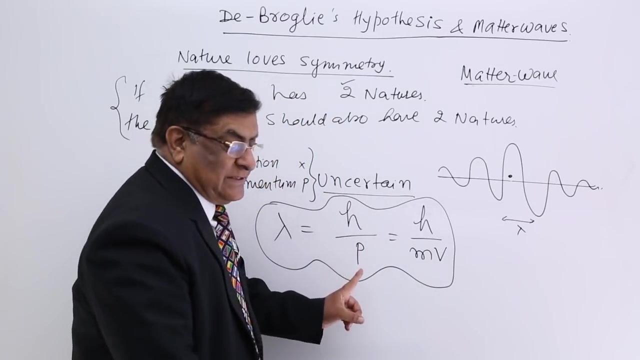 it has a velocity, mass velocity- then it will go in the form of waves. and what will be the wavelength h upon mv? that will be the wavelength, The wavelength of matter. wave may change from 0 to infinity. So first remember this. 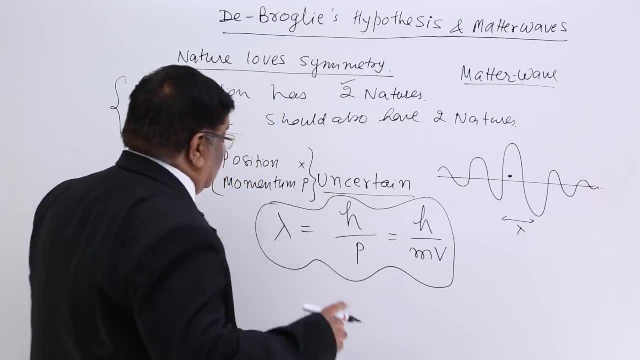 This is de Broglie's equation And this wavelength is known as de Broglie's equation, So first remember this: This is de Broglie's equation, So first remember this: This is a wave and this is a mass. 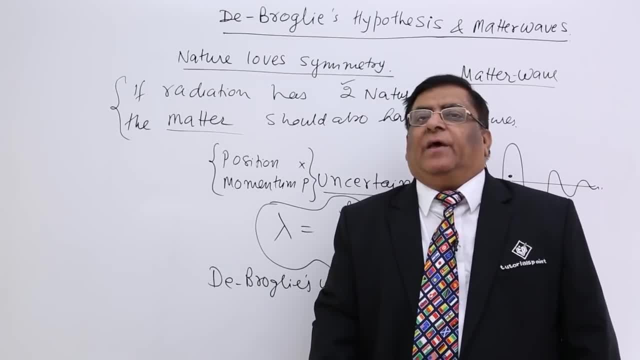 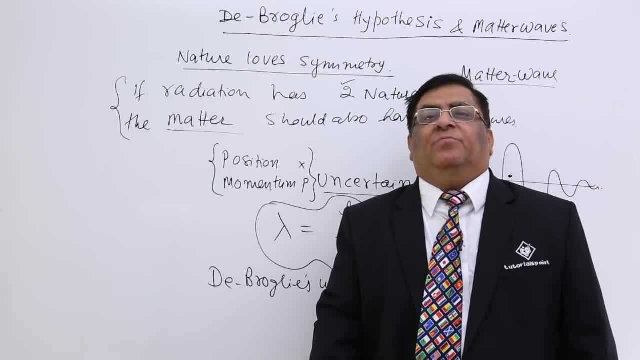 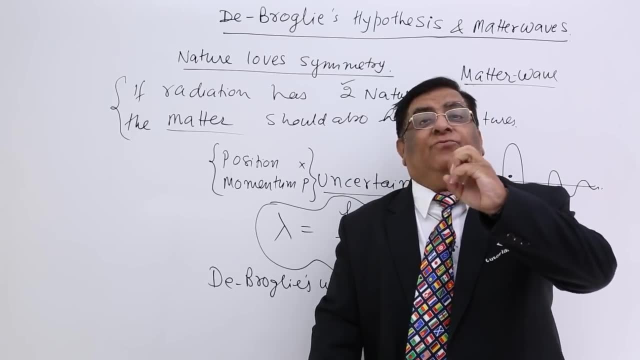 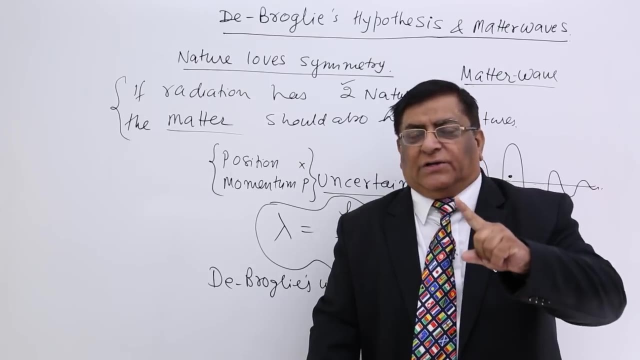 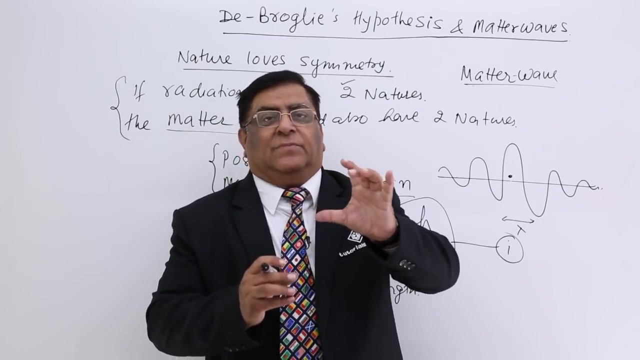 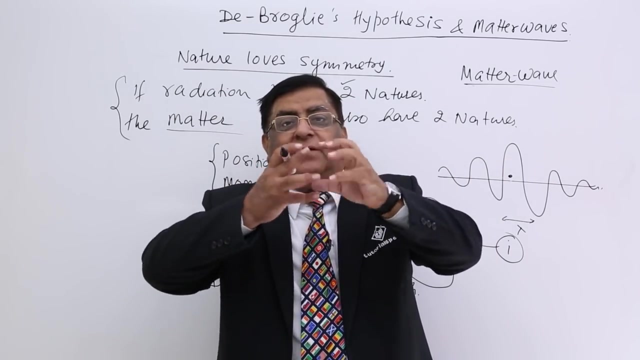 A moving matter, sometimes behave like a material and sometimes behave like a wave. It is enclosed and guided by many waves, known as matter waves. Many waves means why? Why not one wave? Because there is a group of waves, many waves, some small, some large, some small, some large, and all these waves make a group. 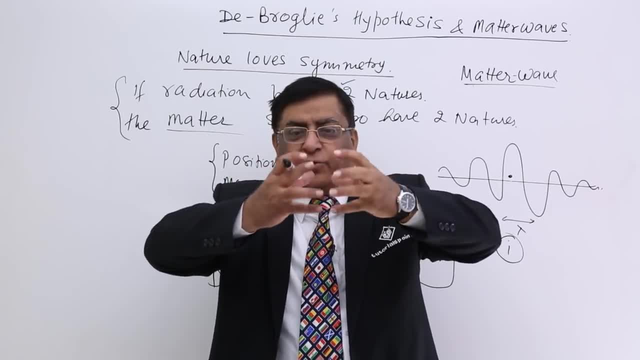 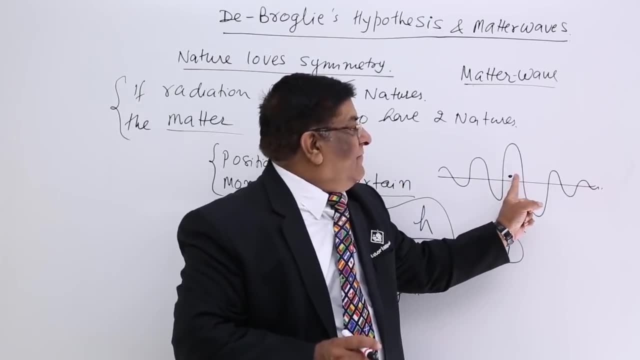 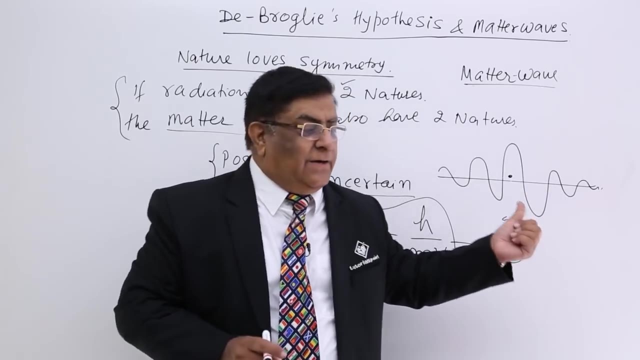 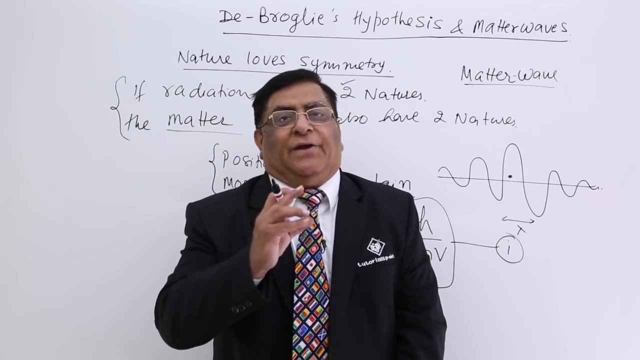 and in that group- it appears to be a group like this- so many waves together and in that group that material is located somewhere, it has a position somewhere, its position and its momentum are uncertain. okay, So that is matter wave, and it always with the material. 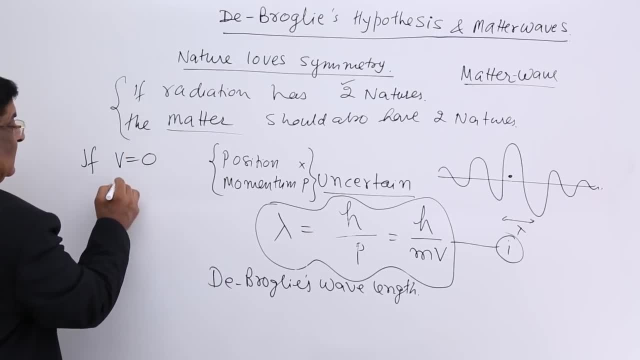 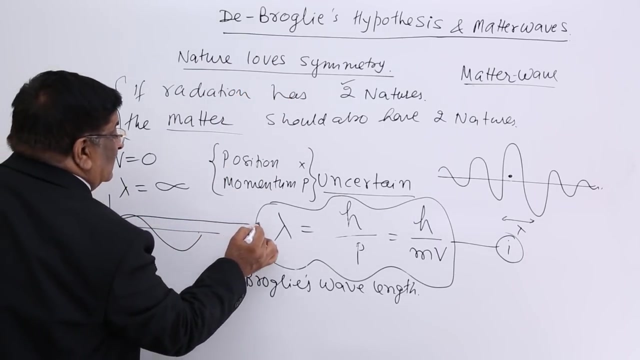 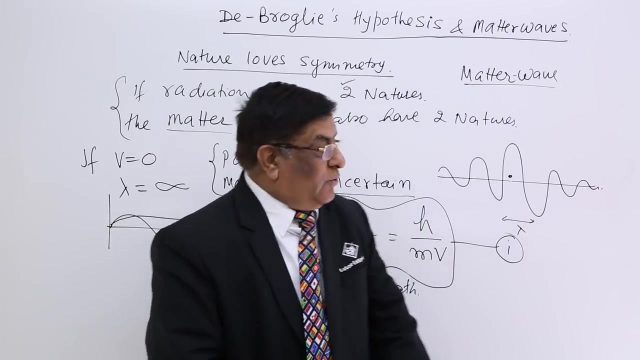 Now, if velocity is 0, then wavelength is infinity. What is infinity wavelength? You see, this is wavelength. Increase it to infinity, then this will go like this: This and the wave nature is gone. That means it does not exist. So if velocity is 0, then 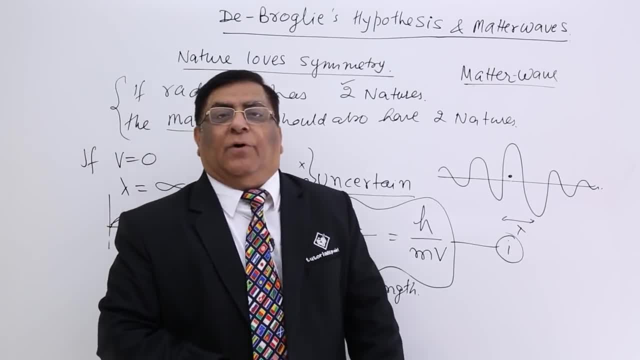 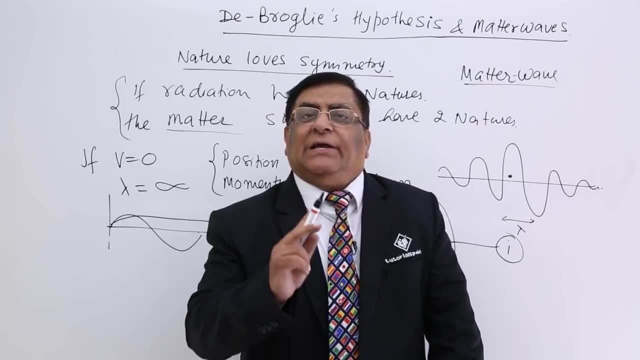 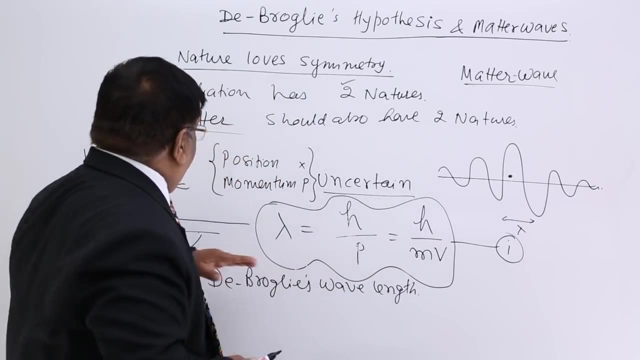 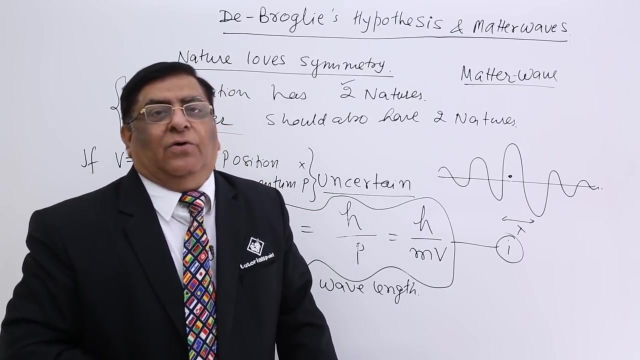 it does not move, it does not travel in the form of wave, it is a matter. So this matter wave exists only and only when the particle is moving. If the particle is not moving- 0,- then wavelength is infinity and the material does not have wave nature. Okay, Now if the 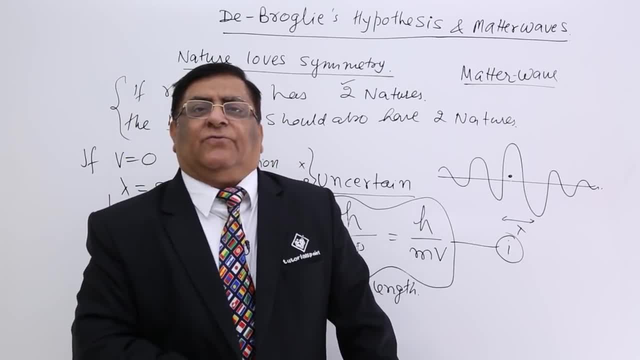 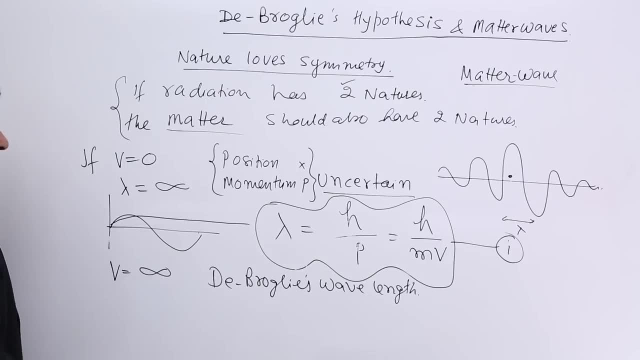 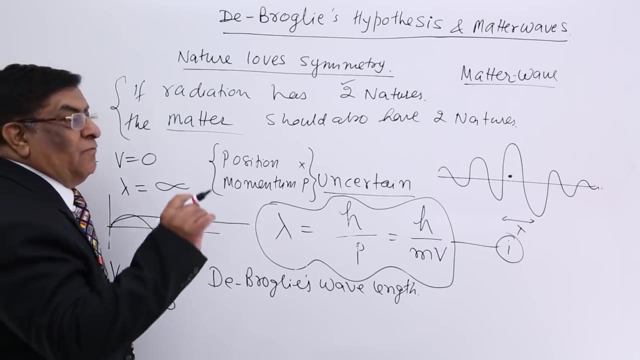 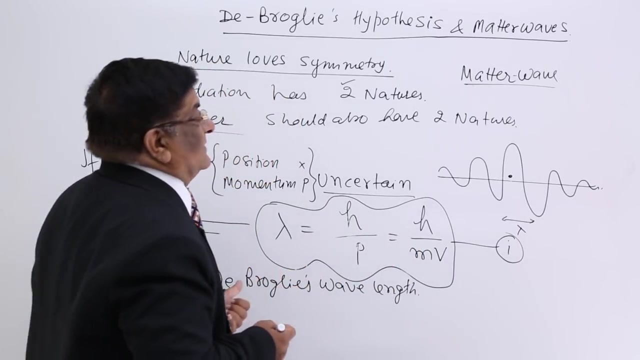 velocity is very fast, just like photon. If the velocity is infinity, if velocity is infinity very large, then what is the wavelength? Very small, Wavelength is so small that the moment that it is difficult to see this. If the wavelength is very small, then it will be like this: 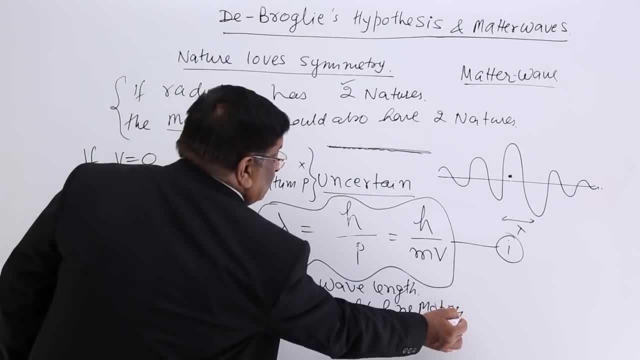 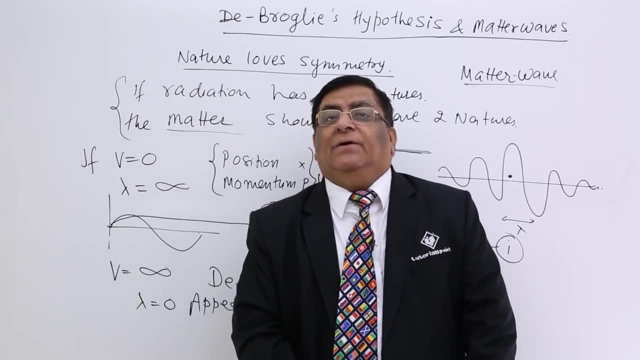 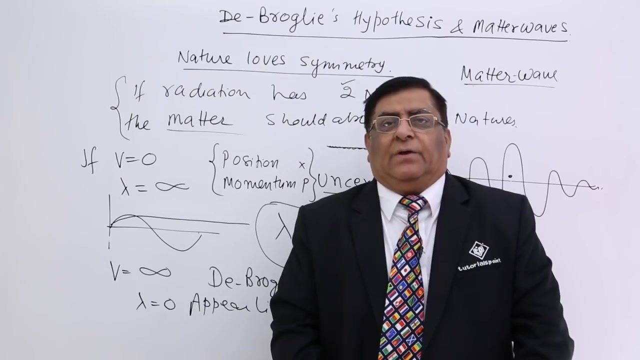 And it will appear like a straight line, line motion. And this is what happens with photon. Photon has a very speed- speed of light very fast- so it appears to move in a straight line. ok, So this was de Broglie's hypothesis and this was the matter wave which is enclosing 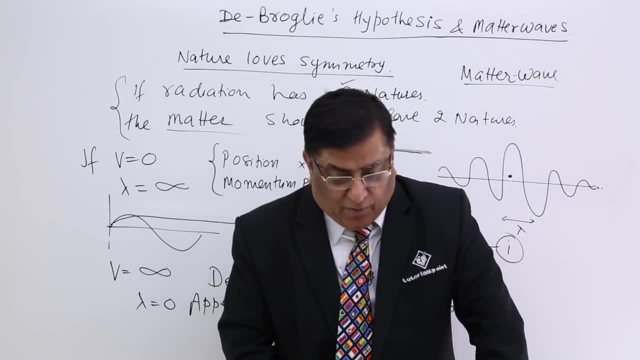 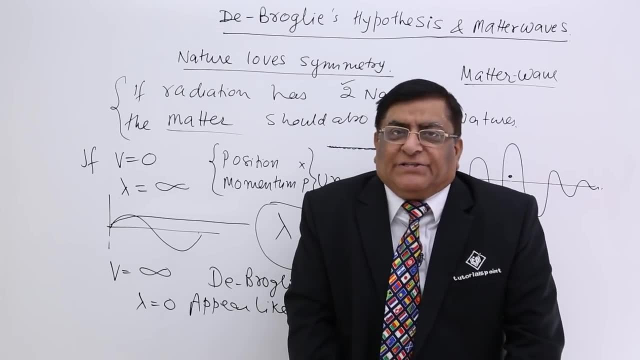 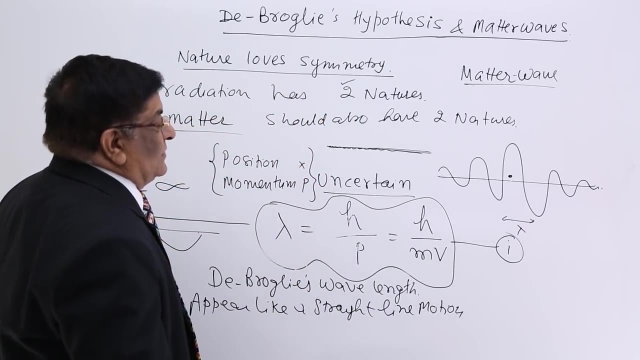 any matter which is under motion Now, this de Broglie's wavelength. is it related to temperature? Answer is yes, it is related to temperature, How it is related to temperature. So for relation to temperature we have to derive it a little bit with energy Now, energy of a particle or energy of a gas. 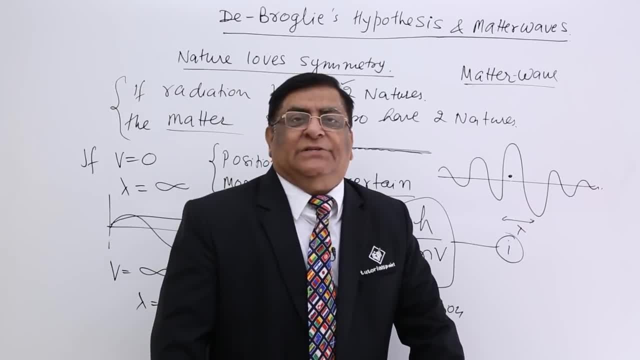 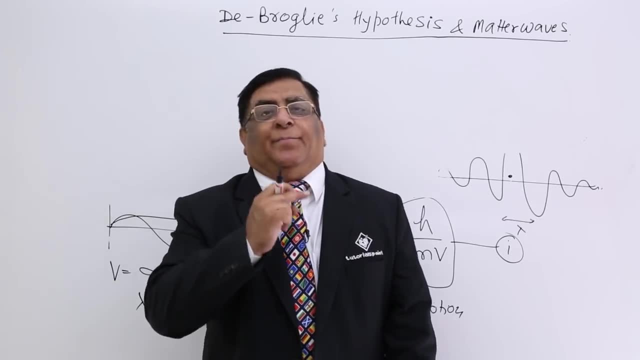 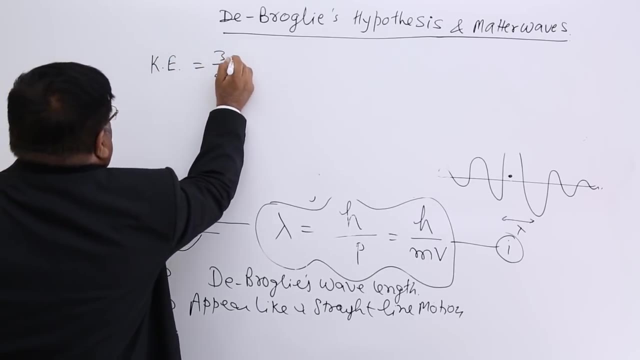 particle is given by an equation which is 3 upon 2 kT. Now we will study the relation of de Broglie's wavelength with temperature. We know that kinetic energy of a molecule is given by 3 by 2 kT. 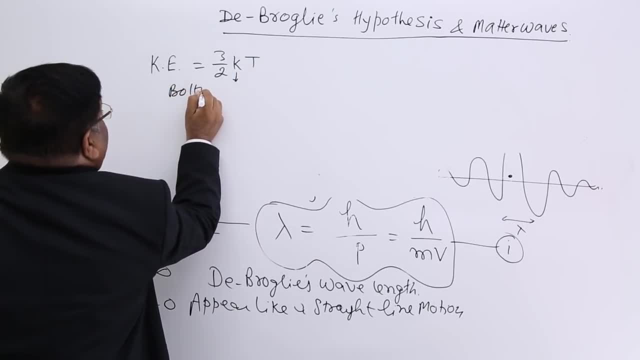 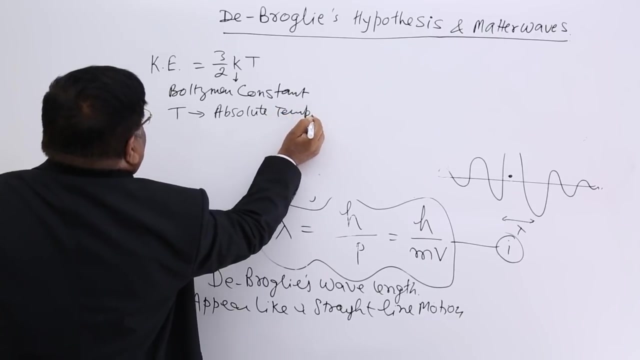 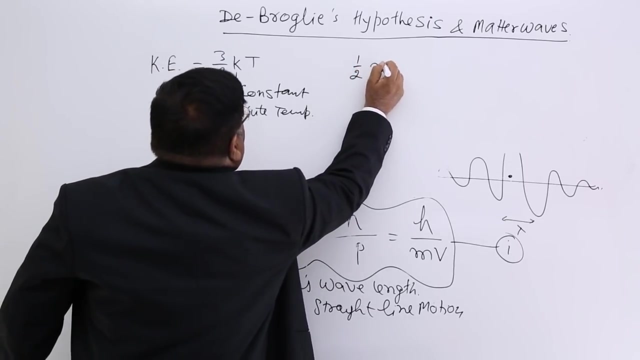 So here 3 is infinite, where K is Boltzmann constant and T is absolute temperature. absolute temperature, Now kinetic energy, is also equal to half mv square. so half mv square is equal to 3 upon 2 Boltzmann constant. Answer is yes. it is given by 3, by 2 kT. Now kinetic energy is also equal to half omv square. So half omv square is equal to 3 upon 2 Boltzmann constant. as I spoke about Europeans night, 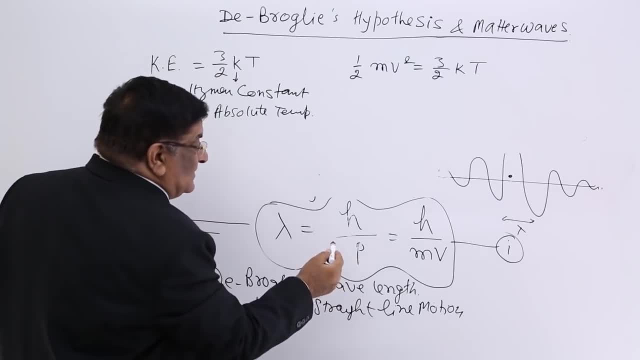 until this, This is your how we will design energy to complete a circuit within a single into absolute temperature. Now this is lambda and we have this formula for lambda: H is a constant and we want to find out value of mv or p. So here mv square, so we multiply. 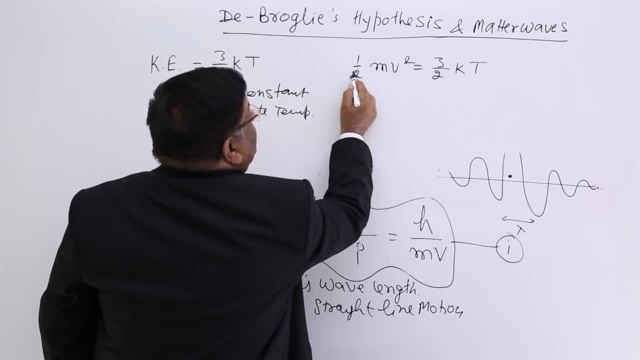 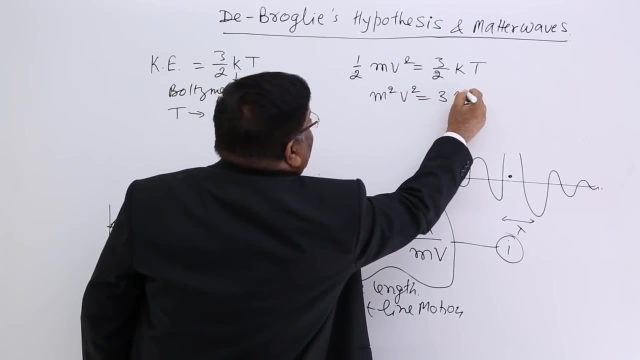 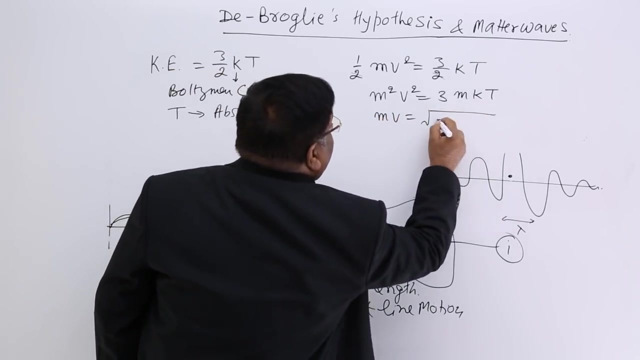 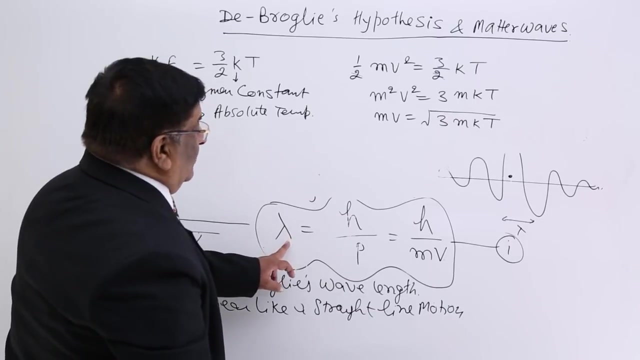 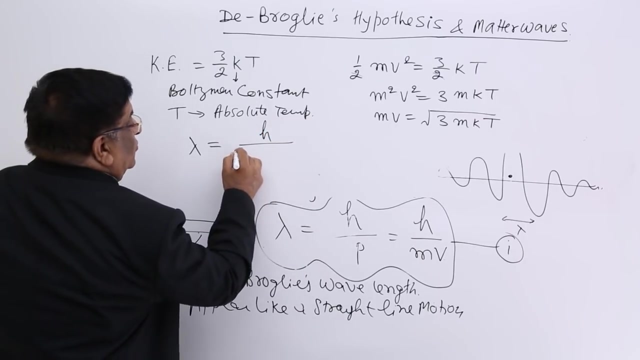 both sides with m and this 2 is cancelled, and this we will make. as m square, v square is equal to 3 mkt. So mv is equal to root 3 m. Boltzmann constant absolute temperature Root 3 mkt. Now we put this value here and lambda is equal to h upon root 3 mass of the. 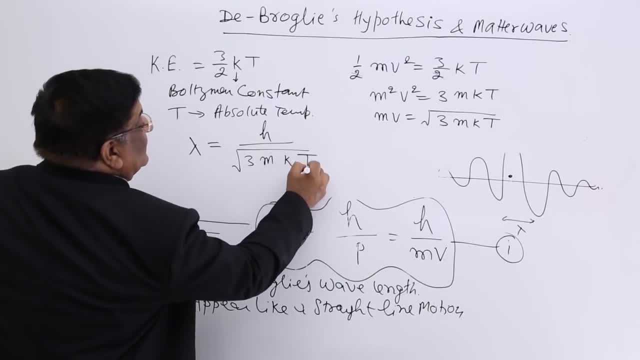 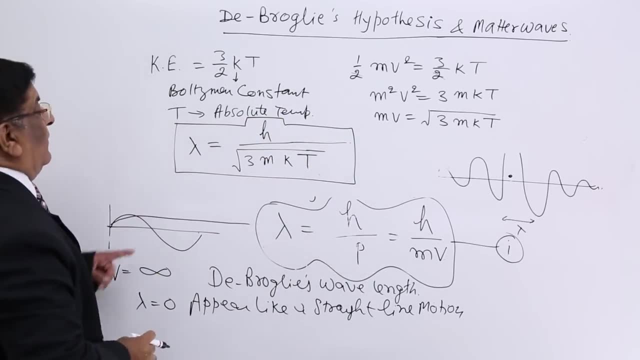 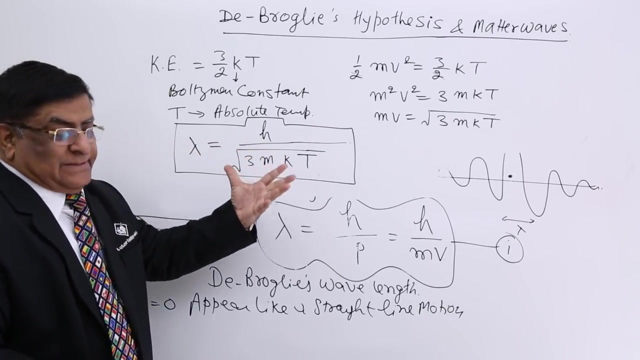 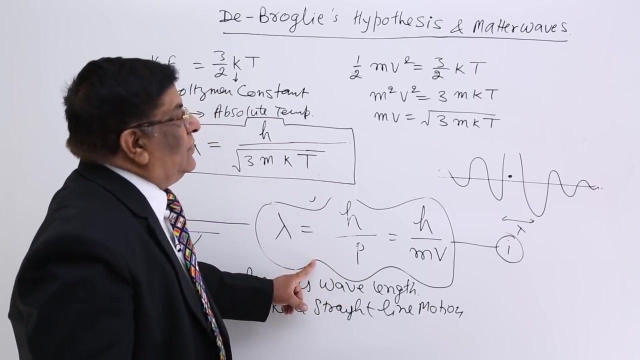 particle Boltzmann constant and its absolute temperature temperature. This is what he predicted should be wavelength, how it is related to temperature. So if the temperature increase, the wavelength will decrease. This is the relation. This is the formula we have done earlier, So now we have got de Broglie's hypothesis Material. 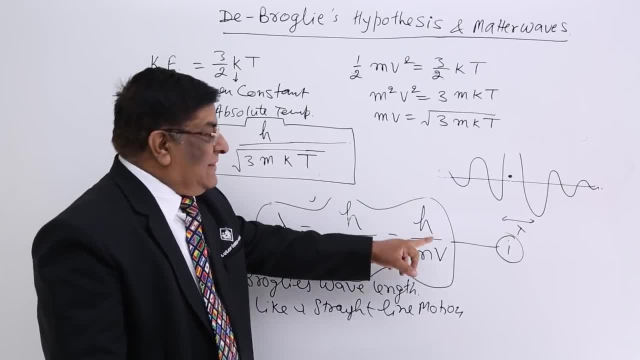 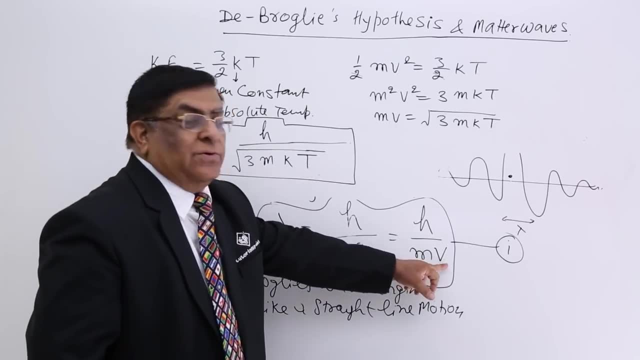 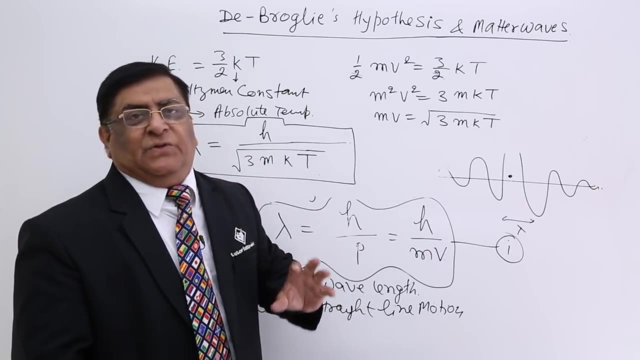 moving has a wavelength. This is the wavelength. We have seen two extreme cases: when v is infinite and when v is 0, there is no wave nature. So wave nature is only there when there is velocity. The wave nature is very much undefined. It is a group of waves enclosing the matter. 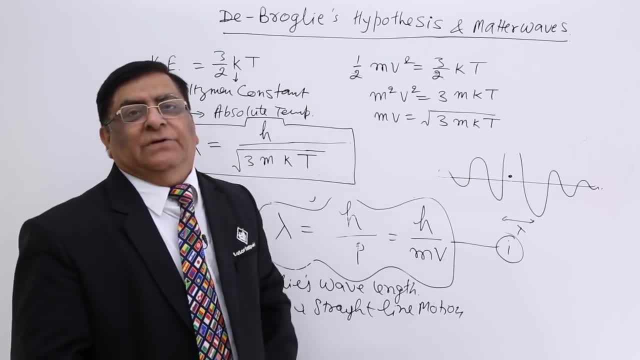 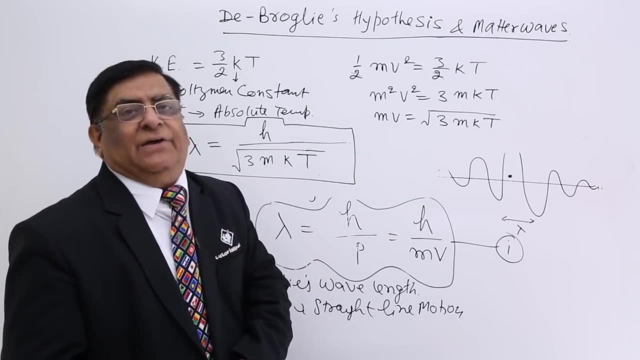 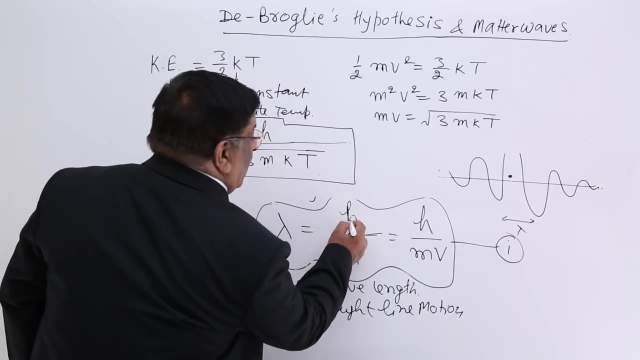 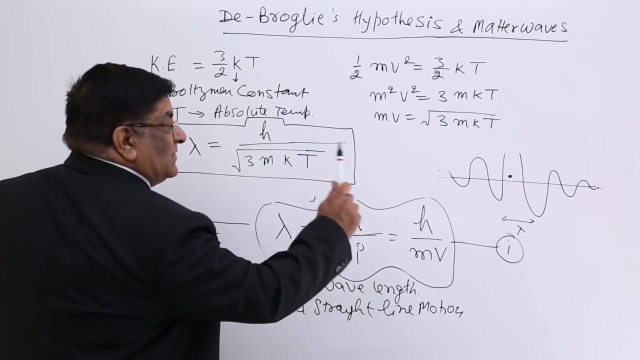 and the matter is guided by that wave. Sometimes it behaves like material, sometimes it does not. waves like waves and this wave has got a wavelength and the formula for wavelength is h upon p. that was the formula for wavelength of the photon. the same way it is h upon p, but because 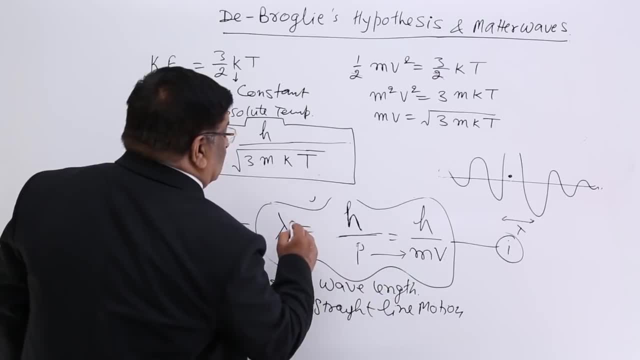 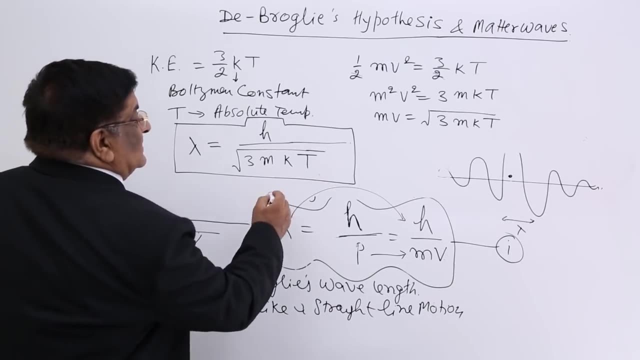 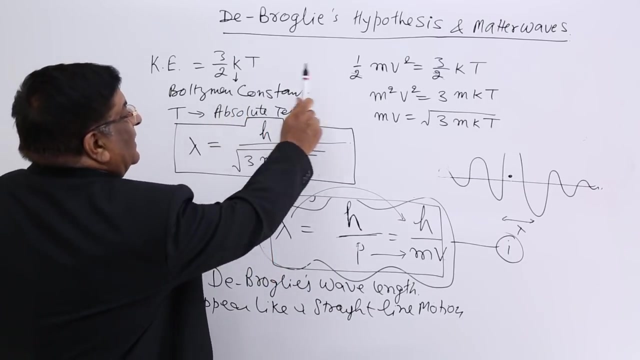 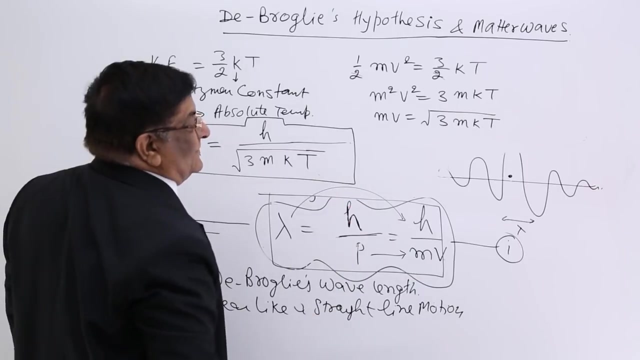 it is a material, p is m into v. so for matter wave h upon m, v is the formula for wavelength. this is de broglie's formula. in the second part we have done that. the wavelength is also affected by temperature. by this derivation, if the temperature increase, the wavelength becomes shorter.